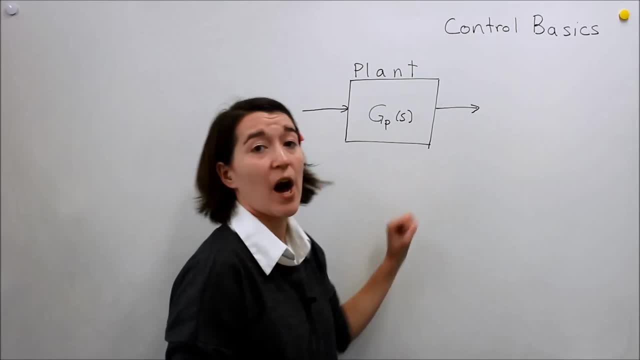 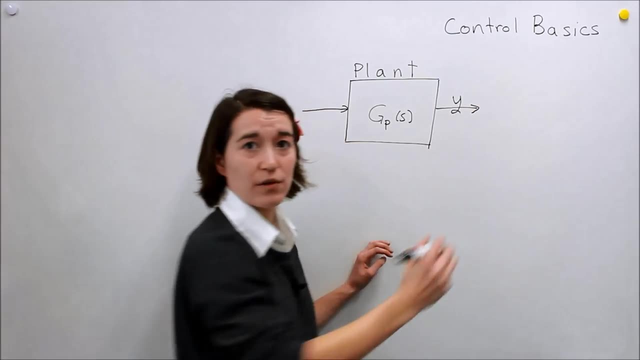 and things like that. For now, we're going to be dealing with single input and single output systems. Okay, so you have an output here. I'm going to just arbitrarily call it Y. we've been using that quite a bit. So you have a system you have. you can input something into it to make it change. 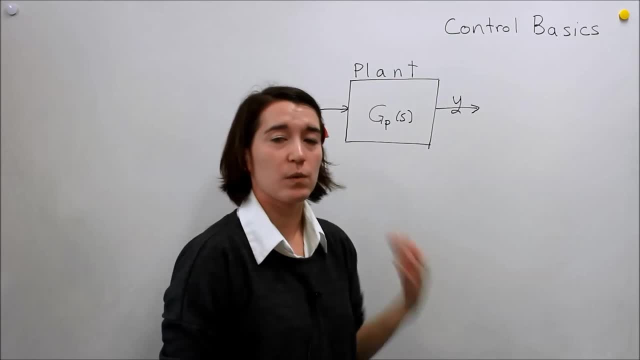 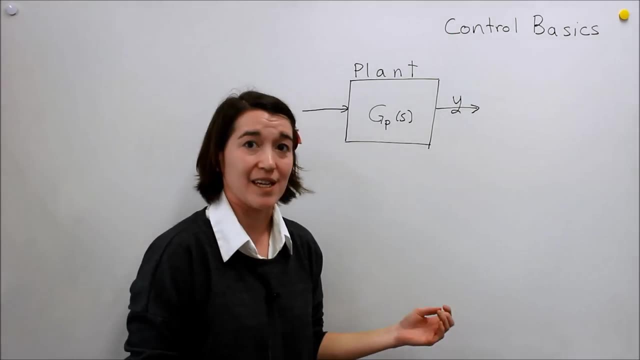 so and that affects the input effects. So that's the input effects that we're going to be looking, the output. But what we really want to do in control is control this output to something We want to make it. for example, if we have a DC-DC converter, a power converter we want 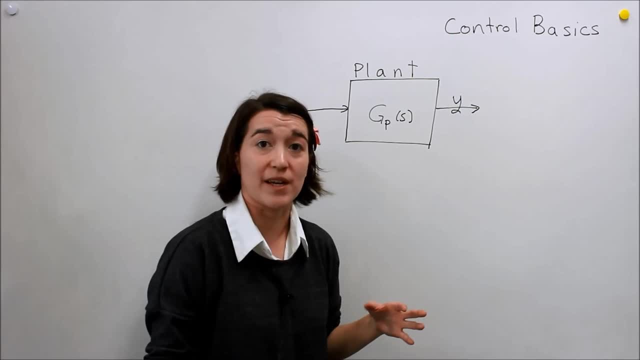 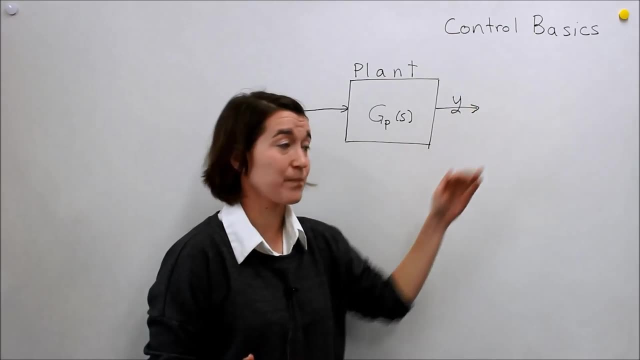 the output to be maybe 5 volts. Say, we're trying to make a USB application, we need it to be 5 volts because that's the standard. If you're flying an airplane, you want to go to a certain altitude, you have a set point of a certain altitude, So you have what we. 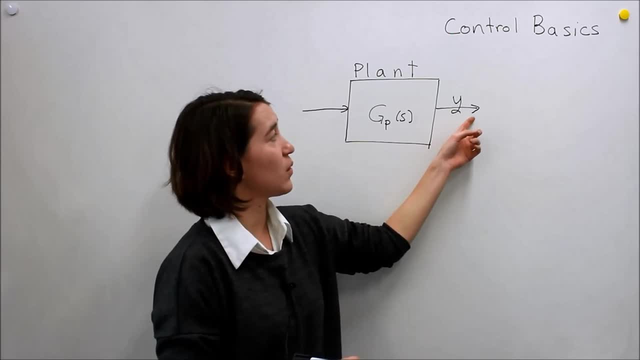 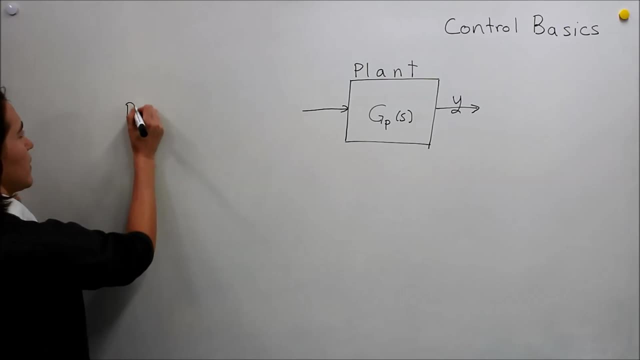 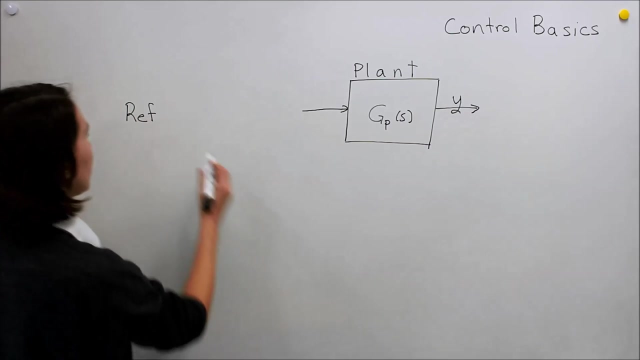 call usually a reference or a set point, and that's usually where we want our output to go to. So we're actually going to write it over here. We're just going to call it reference. If it's a voltage or current, you usually put I ref or V ref here. For now we'll just 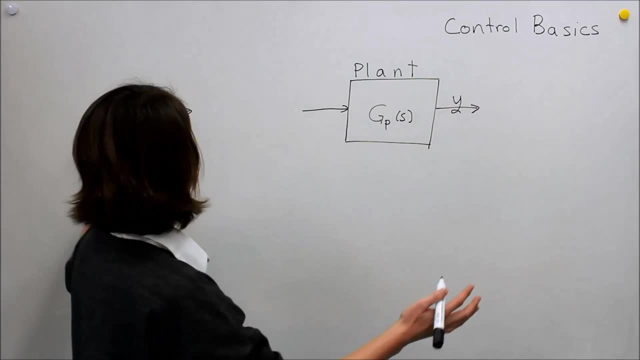 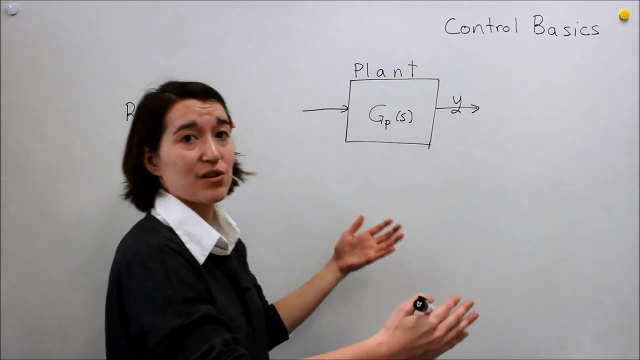 call it the reference. There's a reference value and generally we'll assume that it's a constant. but this constant can also change depending on you know you're changing your system. You want to fly to a higher altitude. you want to fly to a higher altitude. you. 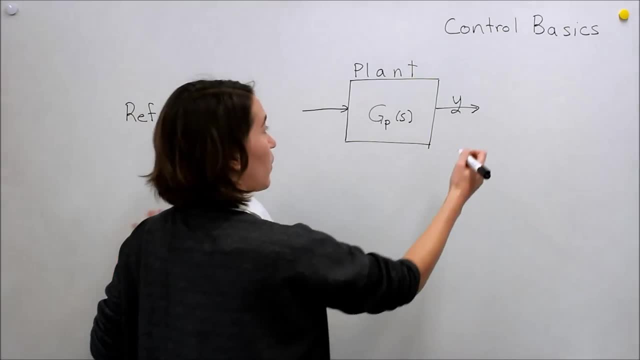 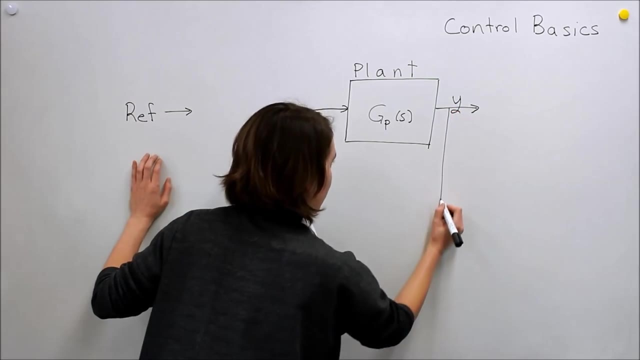 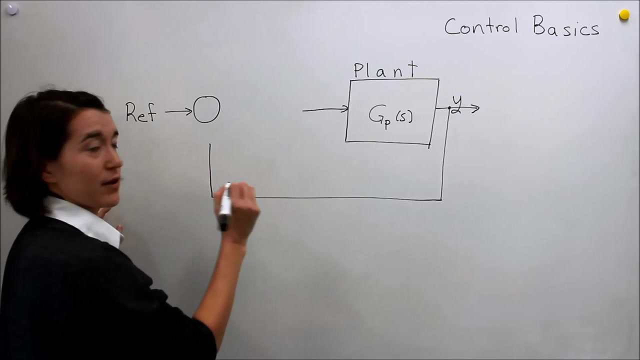 can change this reference, But what we really want is to make sure that Y is equal to that reference. So what we want to do is look at our output and actually compare it to that reference, right? So if it's at the reference already, so usually you do plus the reference. 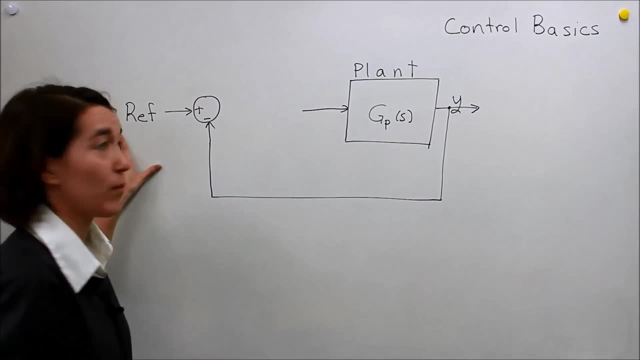 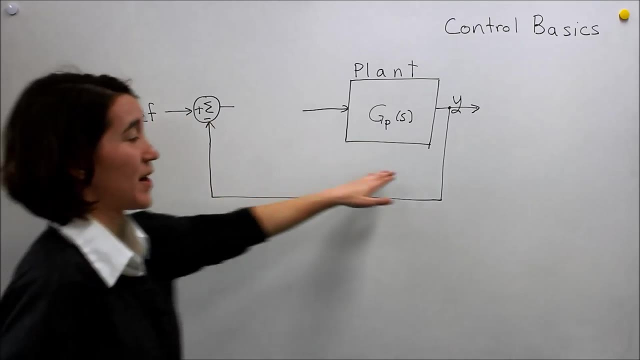 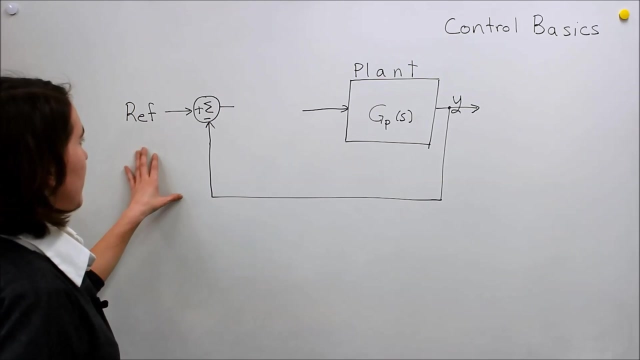 and minus this value. So if they're exactly at the same point, this is a summing block, right? So we take the reference, we subtract the output. If they're exactly the same, it's zero and our system is already set. we're good If it is too low this number. 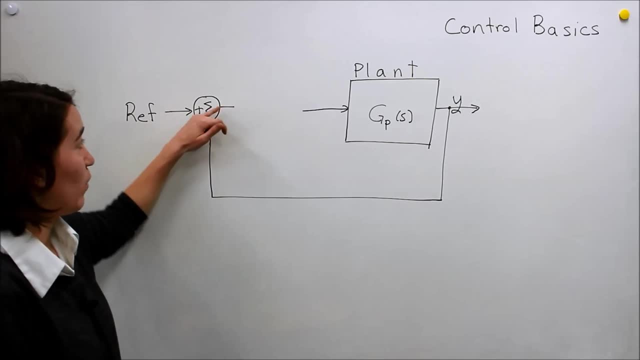 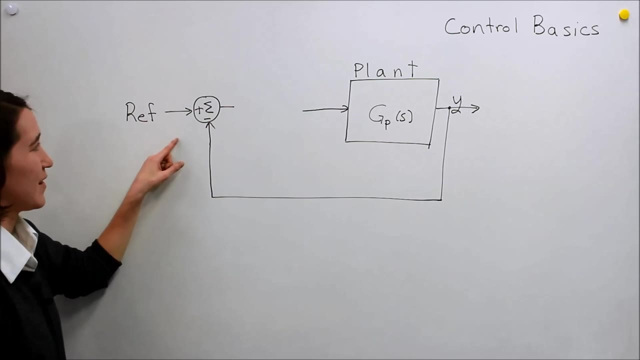 this value coming out here will be positive, right? So then that will feed back into our system here. I haven't connected, finished it yet, but I just wanted to explain the reference difference. If our V out is too high, then we'll have a negative value coming out of.